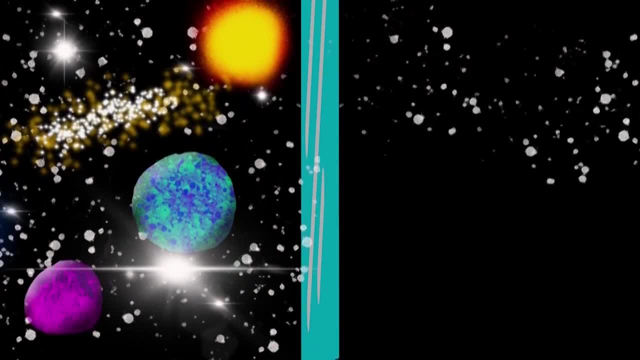 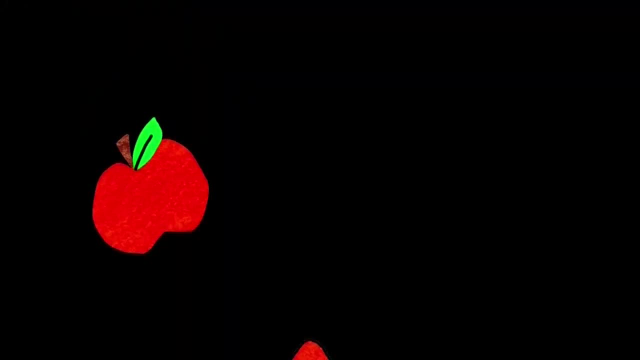 What if we held a giant mirror up to our universe and then built that reflection? Everything is pretty much the same, just flipped. Are the laws of physics, gravity, Newton's forces, magnetism still working the same way they do in ours? If we checked back in a 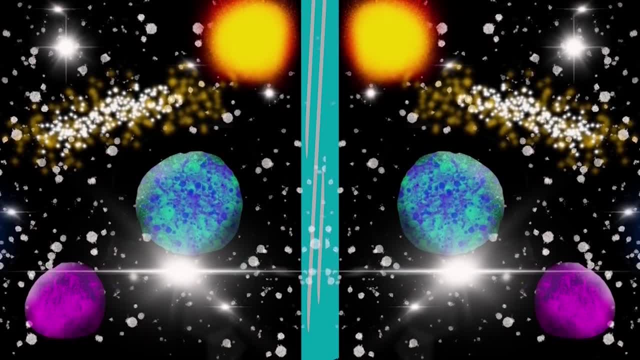 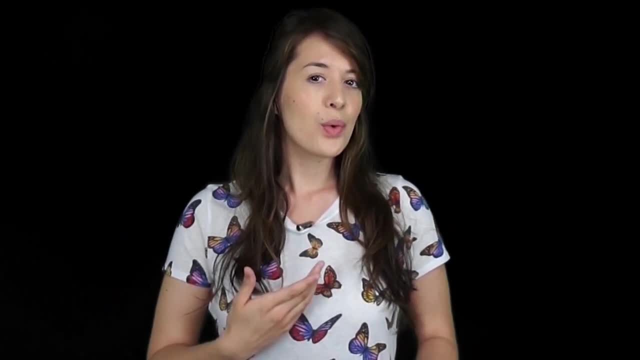 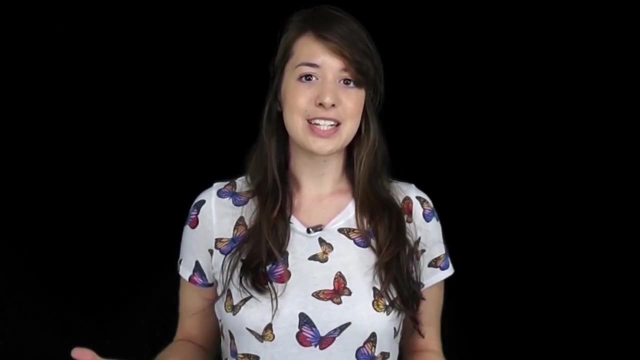 trillion, trillion years, would they still be perfect reflections? This seems like a simple question. Yes, right, If everything is exactly the same just flipped, why wouldn't everything behave the exact same way, just flipped? Well, what does flipping or mirroring something 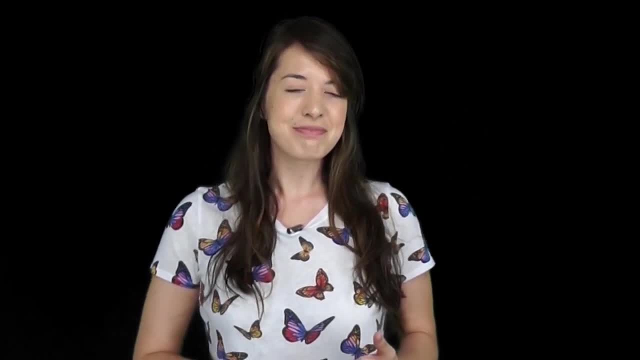 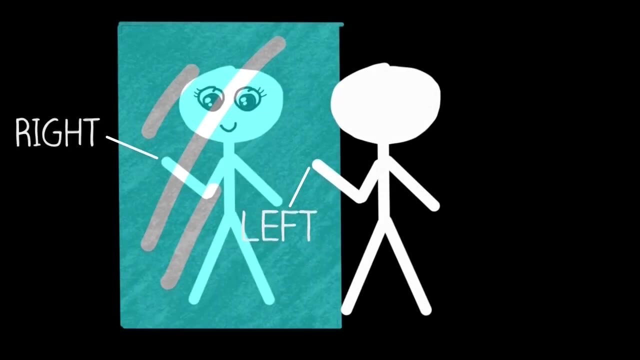 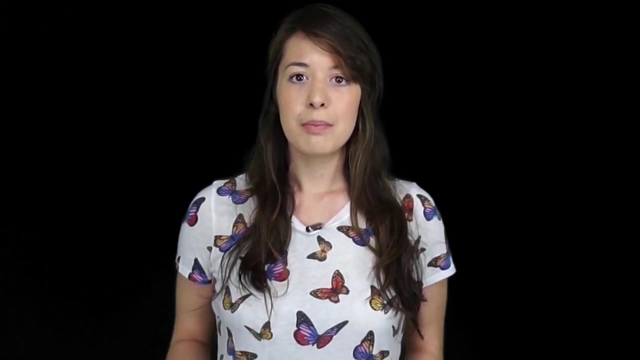 actually do. If you've ever looked into a mirror, you'll probably notice just one difference: Everything that's on your left is now on your right and everything that's on your right is now on your left. This is all. reflection really is swapping left and right, But does. 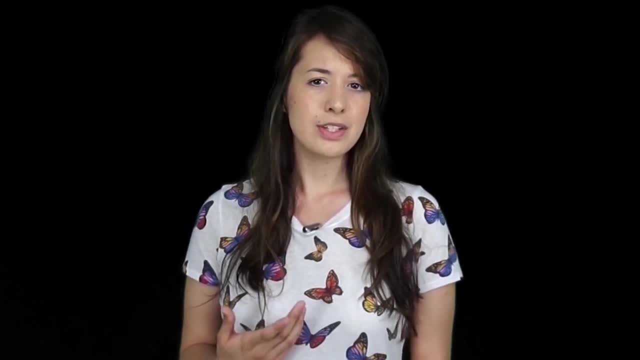 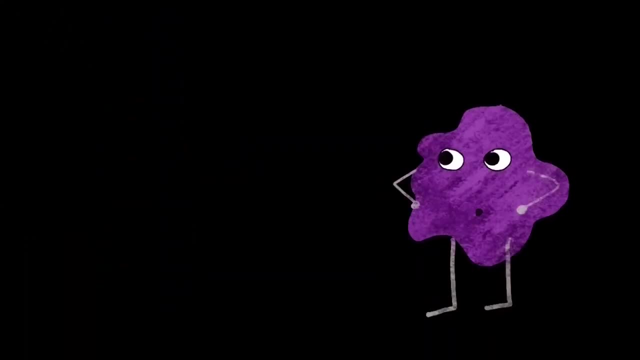 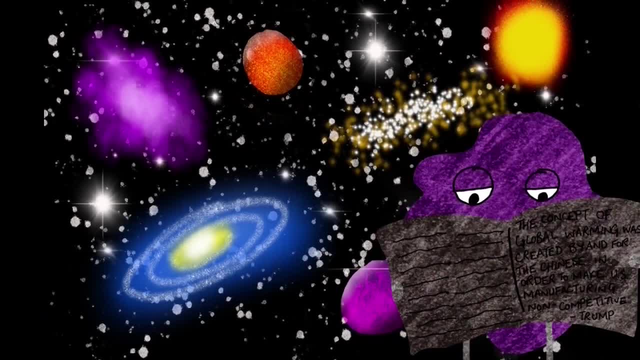 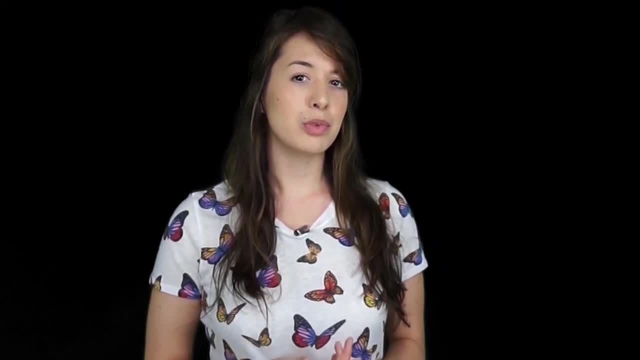 what happened to gravity? This is against the rules. But if left and right were switched? is this breaking any rules? This is kind of a hard concept to grasp and not one we would usually ask ourselves, So I'm going to borrow an analogy from the great physicist and bongo player, Richard. 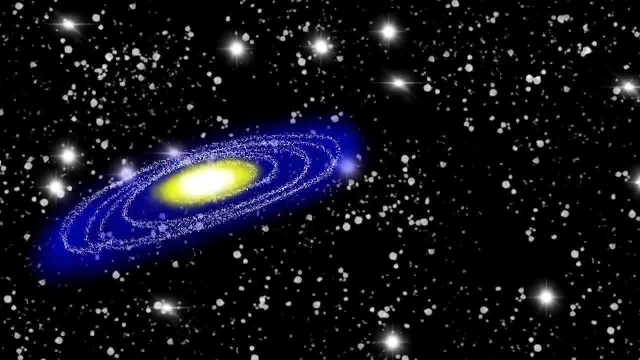 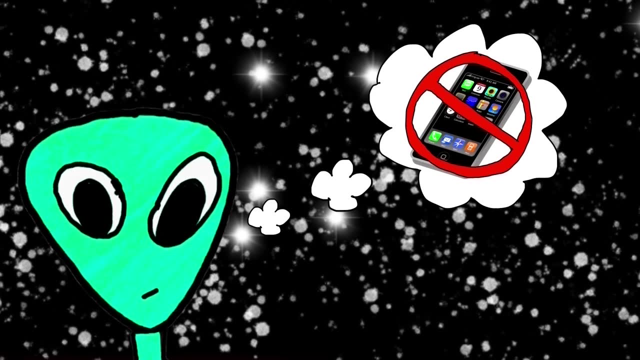 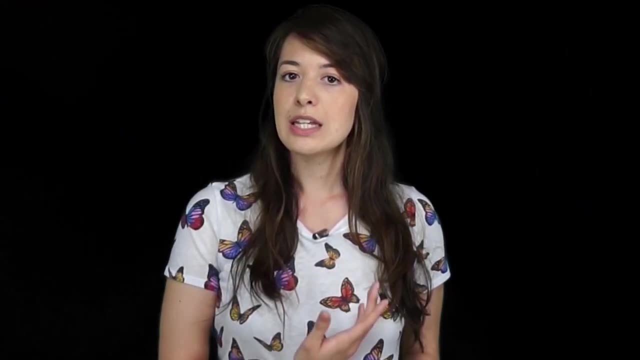 Feynman. He says: imagine you're talking to an alien in a faraway galaxy. Let's call him Simon. Simon is old school and he's not big on smartphones, So sending pictures is out of the question. All you really have in common are the physical laws of the universe. So, if you can, 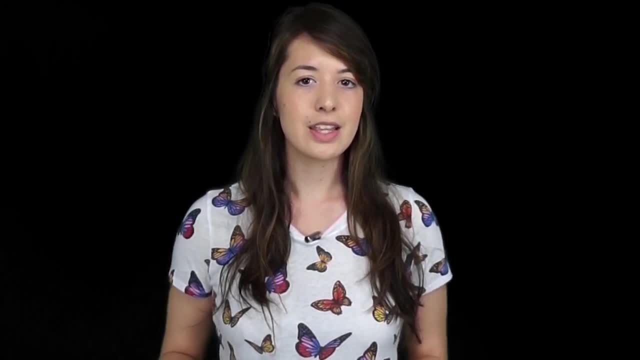 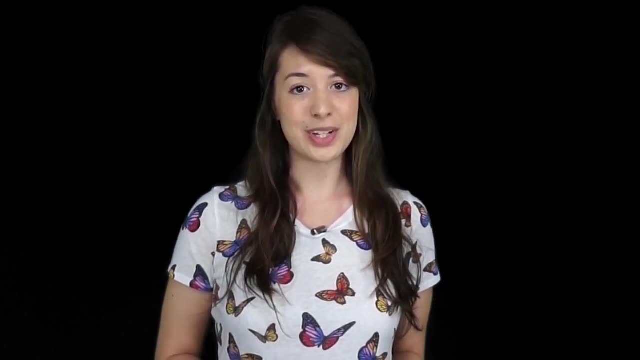 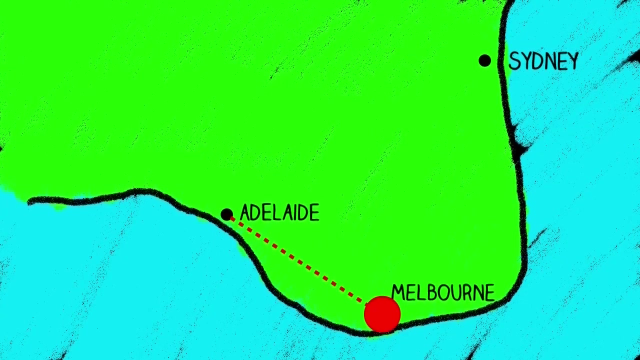 explain to him what left and right are, using only physics, then there must be some kind of rule that says left has to be left and right has to be right. So can you do it? Maybe you'd warm up with geography. If you're standing in Melbourne looking at Adelaide, Sydney is on your right. 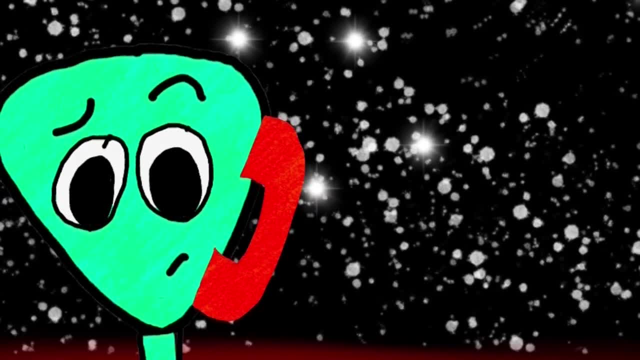 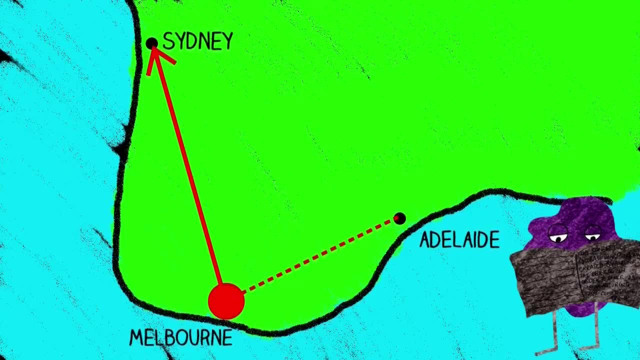 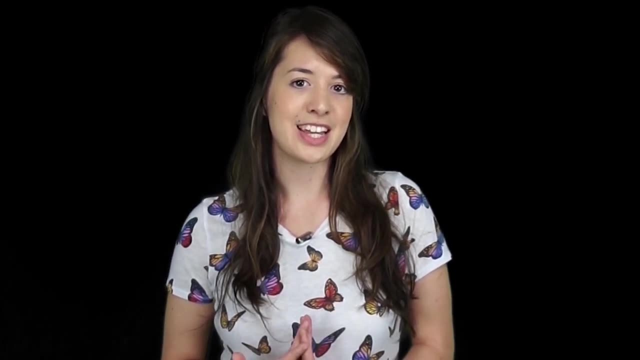 So we can define left and right on Earth, But try telling this to Simon, he'd have no idea what you were talking about. There's nothing in the laws of physics to say that Sydney couldn't be to the left of Melbourne. Defining left and right by geography is just convention invented by us humans, and 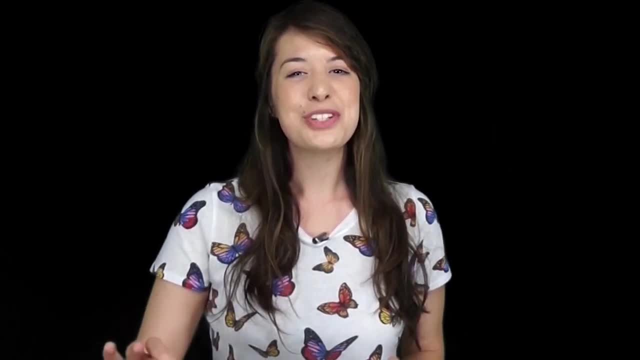 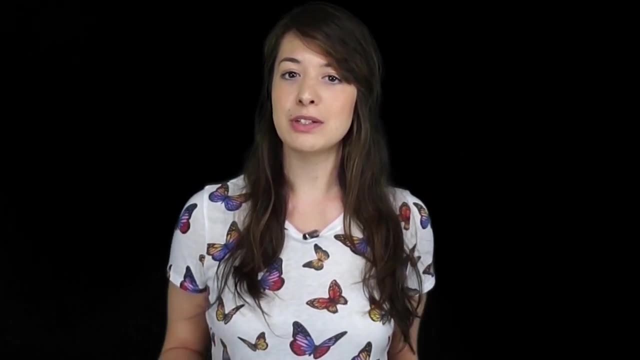 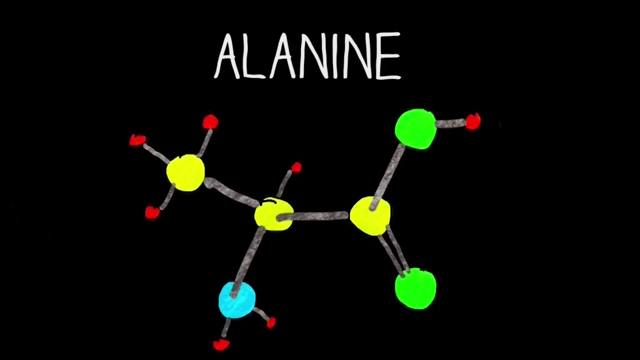 doesn't mean much to Simon. Okay, that was just a warm up. A better example that seems to distinguish between left and right is life. Amino acids are the building blocks of life, and one that shows up a lot is called alanine. Amino acids usually have a left and right-handed. 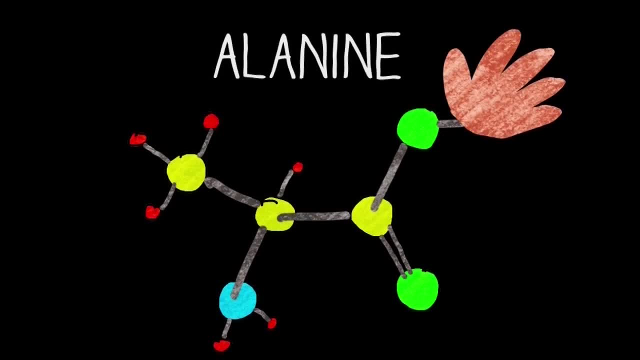 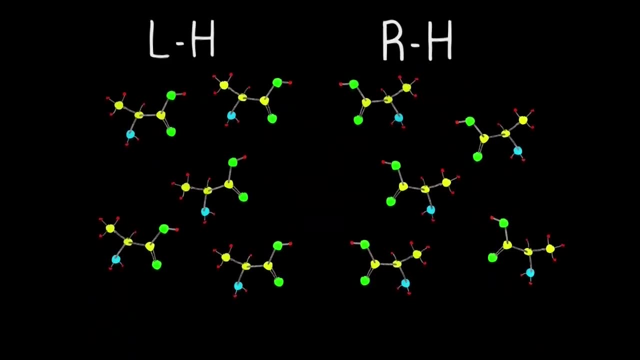 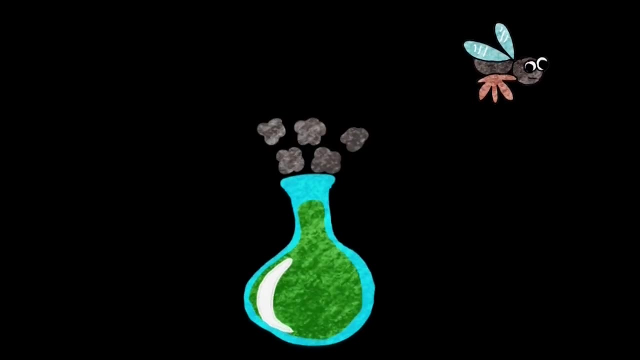 version. but when we find alanine in nature, it's always left-handed. What's even stranger is that when we make it synthetically in a lab, equal amounts of left and right-handed molecules are created, Yet life is all left-handed. So if we bubbled up a synthetic right-handed fly? 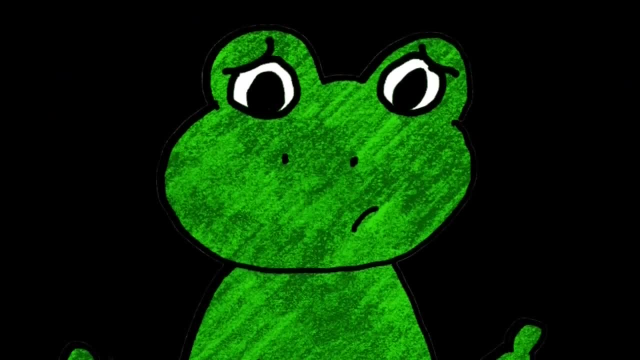 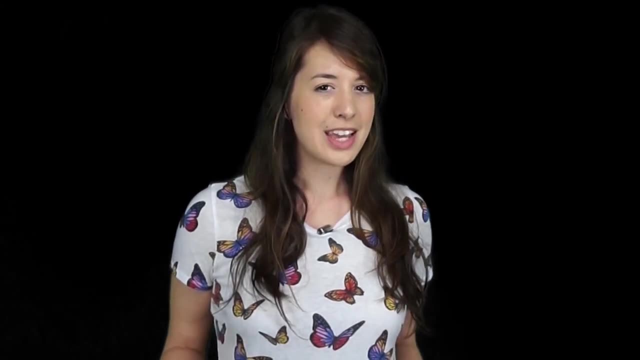 and fed it to a frog, it wouldn't be able to digest it because all of its digestive enzymes are the wrong way around. They're made for a left-handed fly, So it would seem as though life does make some kind of distinction between left and right. So you say: hey, Simon, take a look at. 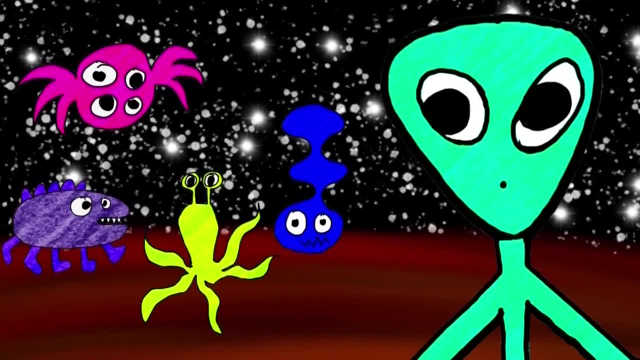 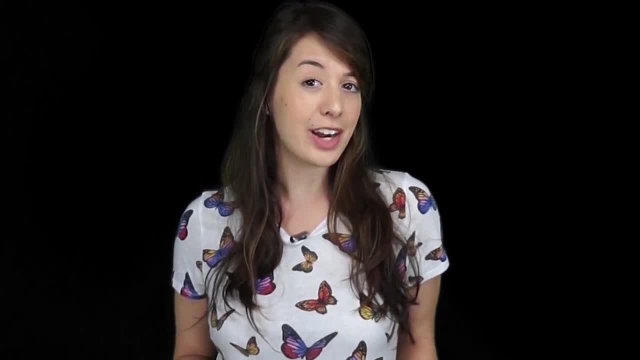 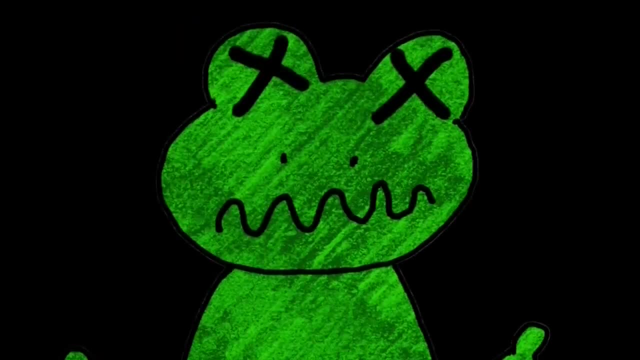 the alanine molecules in life on your planet, Whichever way they're facing. that's left-handed. But wait, is there a reason life on his planet couldn't be right-handed? Our synthetic right-handed fly didn't work, but that's just because of the way it reacted with a left-handed. 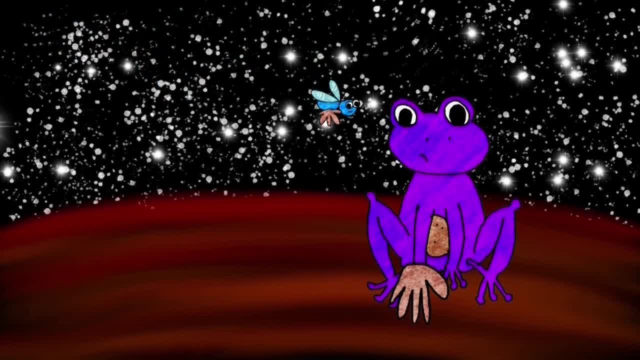 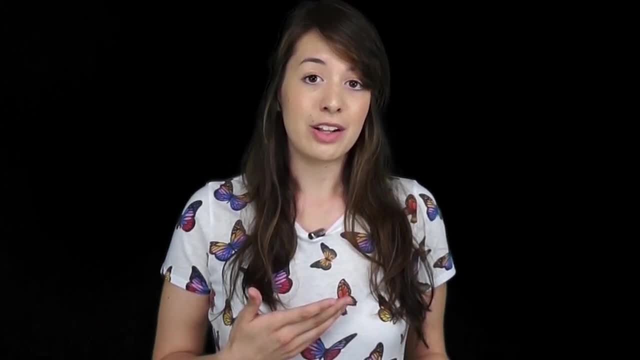 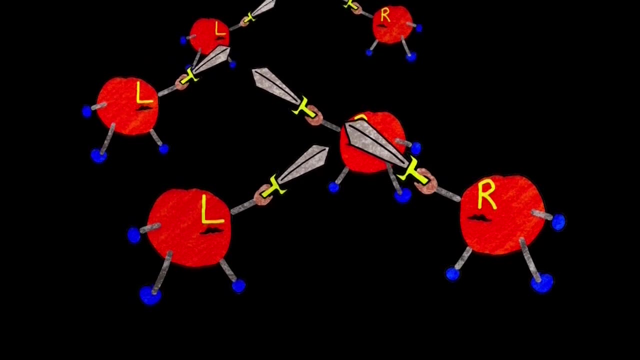 frog. If Simon's planet had a right-handed flies and right-handed frogs, that would work out fine. But didn't we just say all life was left-handed? Well, yes, life on earth. 3.8 billion years ago, when life was first forming on earth, some left-handed molecules just happened. 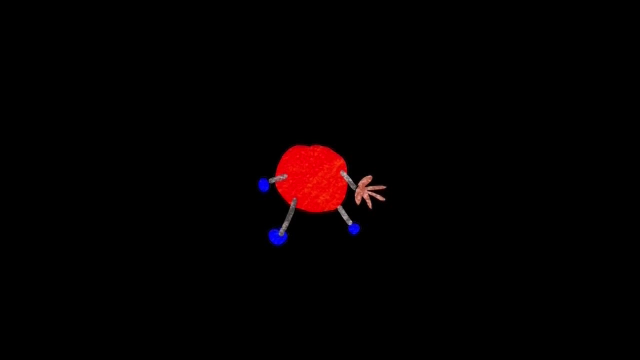 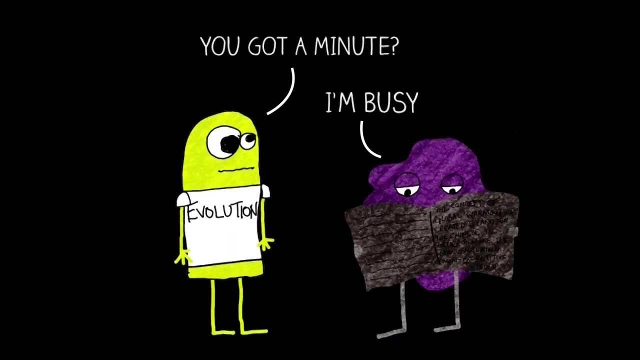 to win over some right-handed ones, And from then on life gradually became left-handed. It could have easily gone the other way, and physics had no say in the matter. It was just pure chance. So if we told Simon that life on his planet is left-handed, there's a 50%. 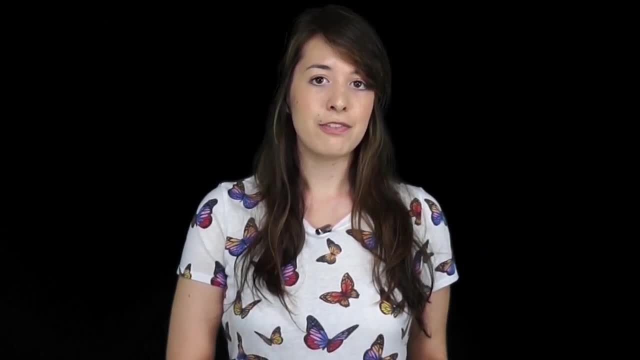 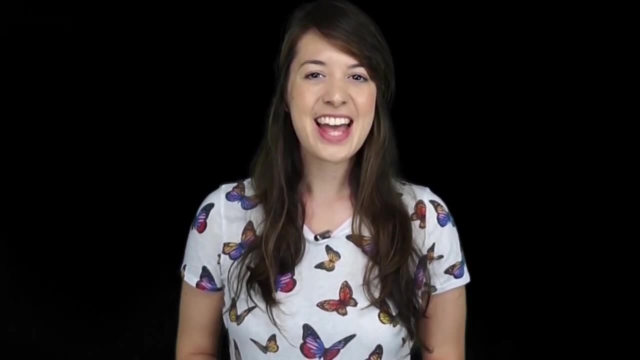 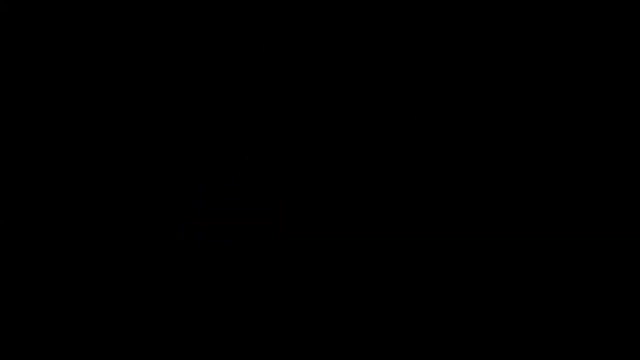 chance we'd be wrong. There's just as good a chance that life on planet Simon is right-handed as there is left. But now we come to something which sounds pretty promising: Left and right in physics. Physics has many left and right-hand rules. For example, if you take a magnet and wrap, 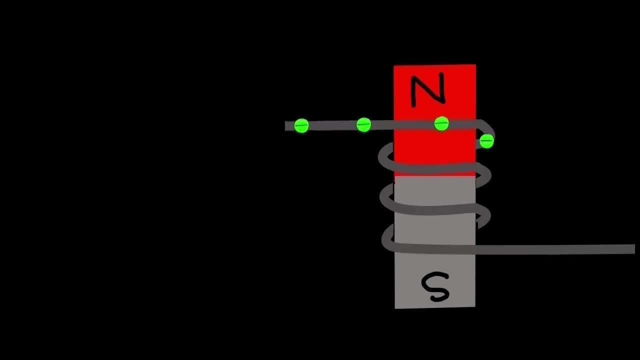 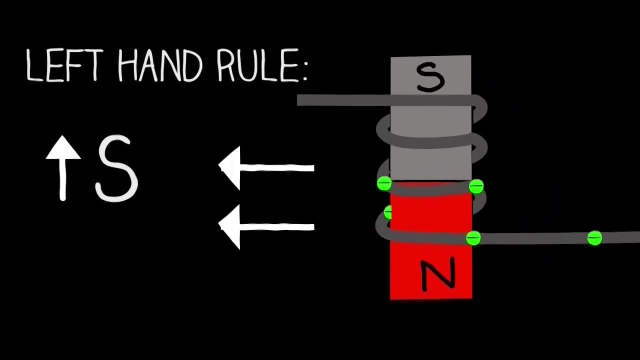 a wire around it, the magnetic field will produce a current through the wire. If the north pole is pointing up the current flows to the right, If the south pole points up the current flows to the left. Magnets are the same everywhere in the universe. Electrons are the same everywhere in. 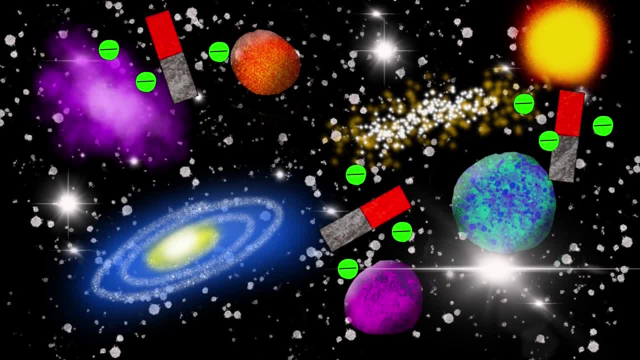 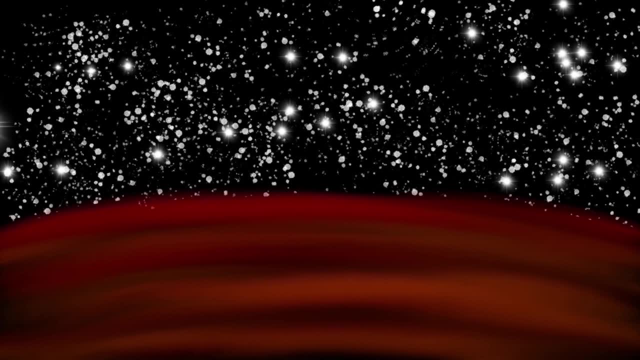 the universe. So the current should flow the same way everywhere in the universe. You tell Simon, find a magnet and wrap some wire around it, Make sure the south pole is pointing up, and then the direction the current flows is left and the opposite of that is right, To which he'll say: 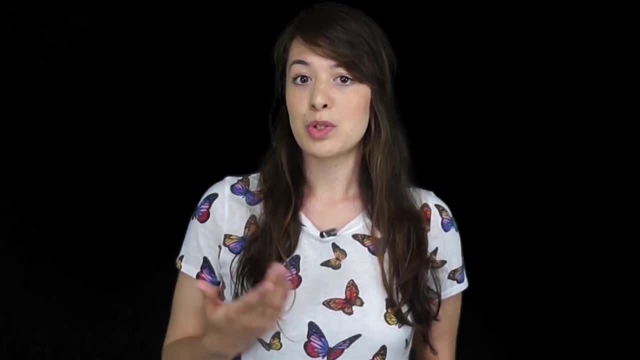 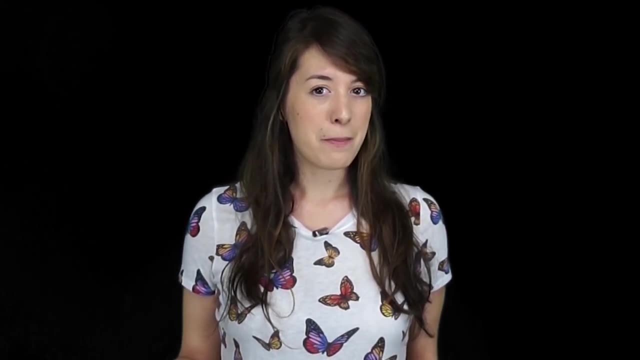 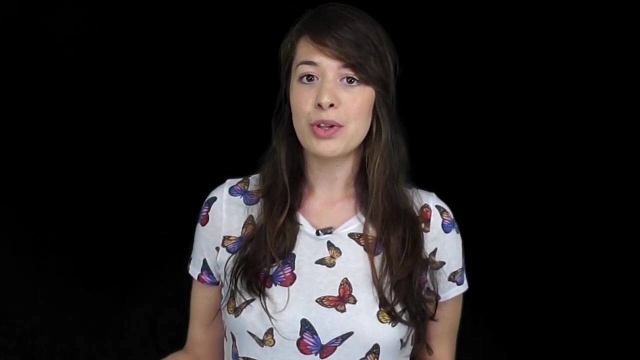 which is the south pole. You could say the difference between the north and south pole is that the north pole points north and the south pole points south, which seems fair. But the thing is that doesn't mean anything outside of Earth. The north and south pole of a planet depend on its spin. The Earth spins. 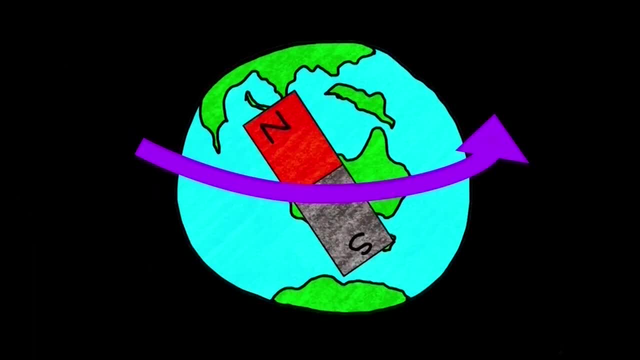 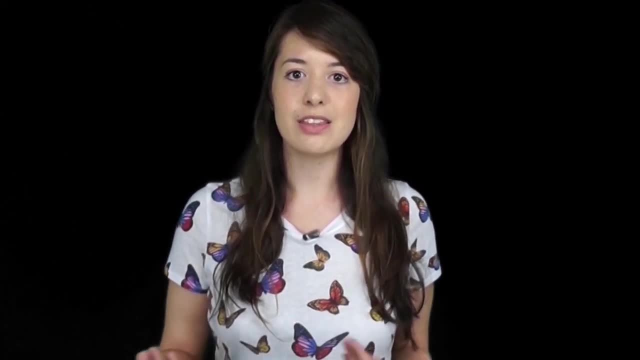 counterclockwise, but if it spun the other way, the north and south pole would be reversed. So let's just ask Simon which way his planet is spinning, Easy right, Then we could tell him what the south and south are and he could figure out left and right from the magnet and wire. 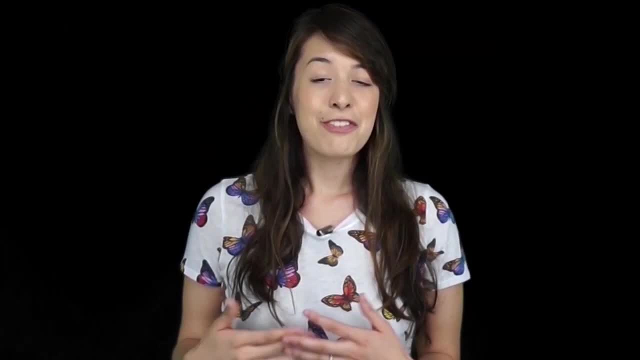 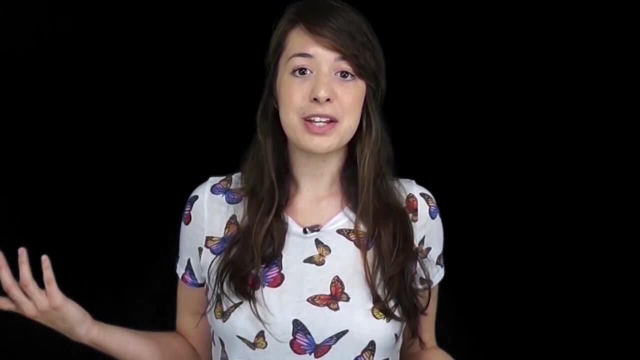 Unfortunately, that kind of leads us back to where we started. If you look closely enough into any right or left hand rule in physics, it always breaks down at some point. What would be a physical difference is if the south pole were growing tiny hairs. 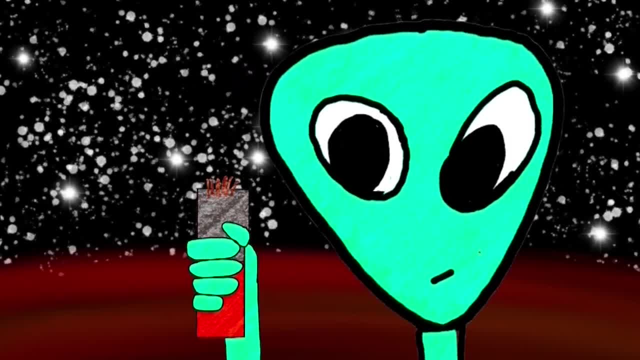 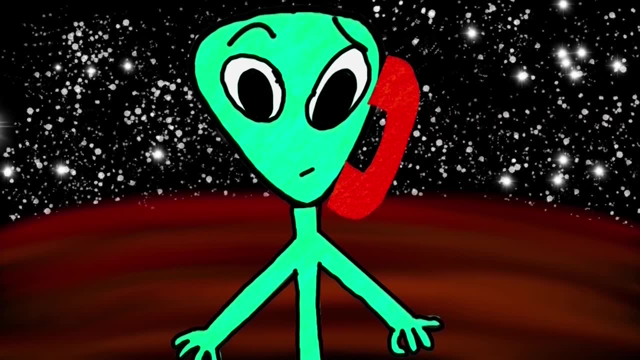 for example. Then we could tell Simon, the south pole is the one with the tiny hairs, and he'd know instantly what we were talking about. But so far we're no closer to telling him. left and right are, and he's getting pretty impatient. 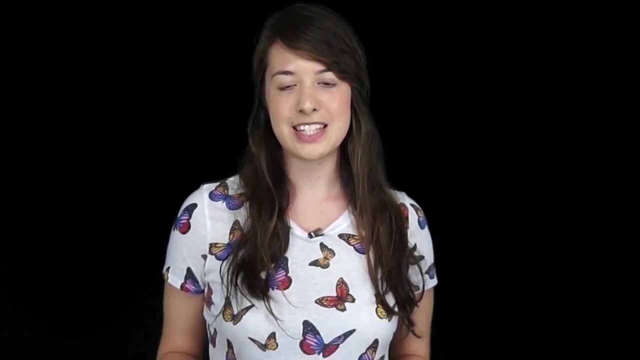 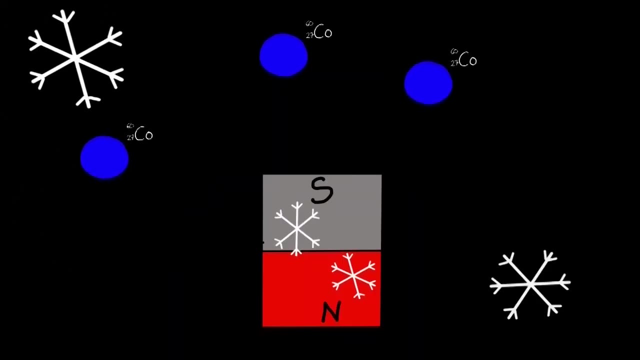 But we've still got one more trick up our sleeve. In the 50s an experiment was performed at the University of Columbia using a very strong magnet at a very low temperature. At extremely low temperatures, it turns out, a certain isotope of cobalt becomes magnetic. 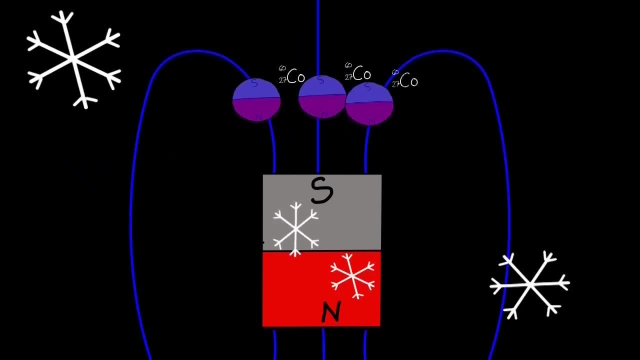 These tiny cobalt magnets will line up in the magnetic field and when they disintegrate, they emit an electron. and it was discovered that the majority of electrons will always fly away from the South Pole. This may not sound like much, but we've just discovered: 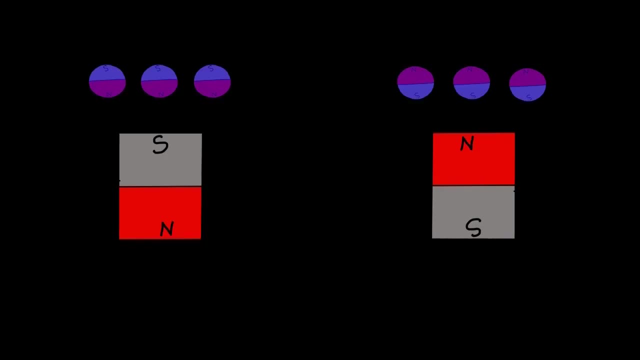 a physical way to distinguish the South Pole from the North. When a magnetized cobalt atom disintegrates, the majority of electrons will fly in the direction away from the South Pole. Basically, the magnet has grown hairs and if there's a physical difference,